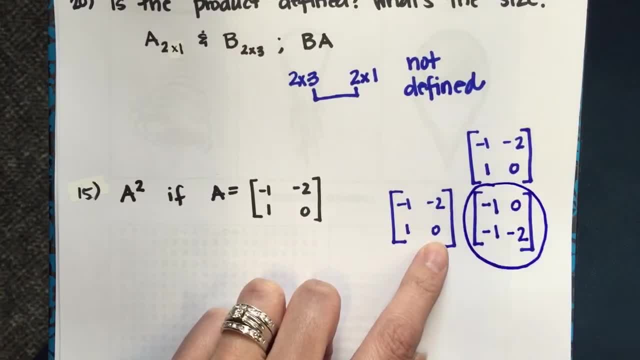 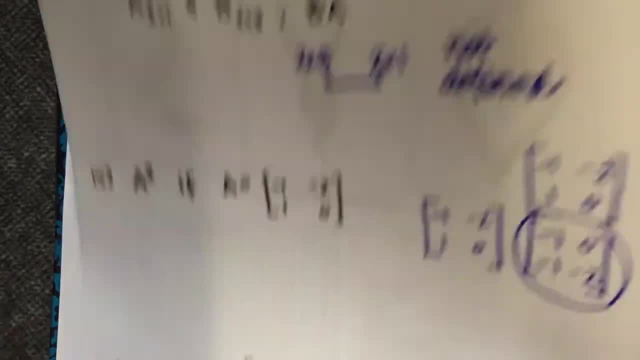 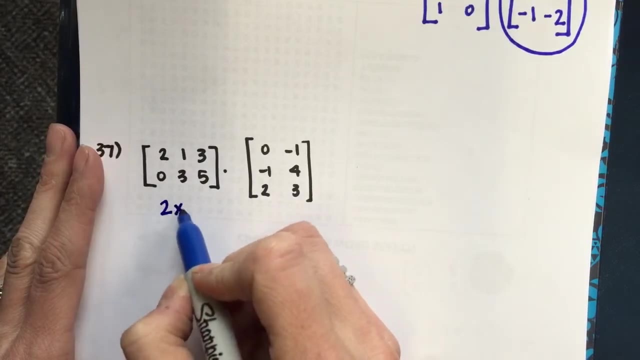 So there, that is A squared. You can see that is not just squaring each number. The last one, number 37.. Multiplying these two matrices, This one has two rows And three columns, It's a 2 by 3.. 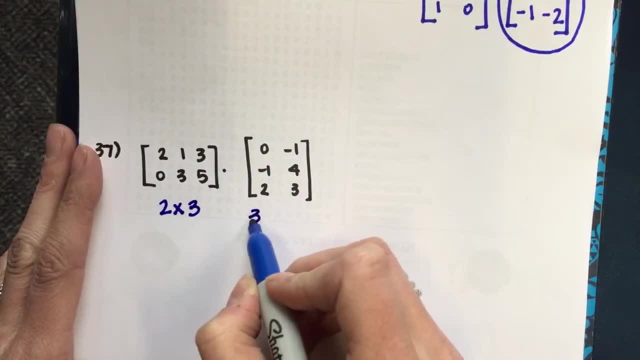 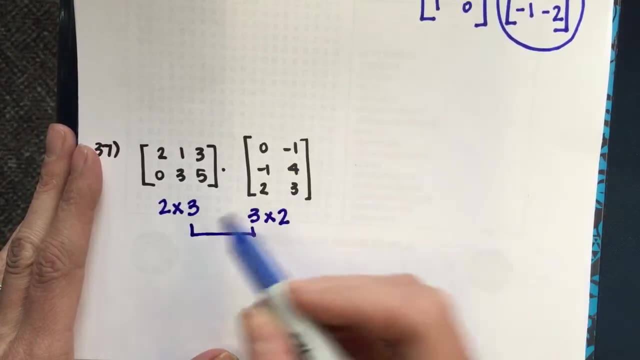 This one has three rows By two columns. We check to make sure the product is defined. Those match And it is The answer. the product matrix will be a 2 by 2.. So when we set them up, this one goes first. 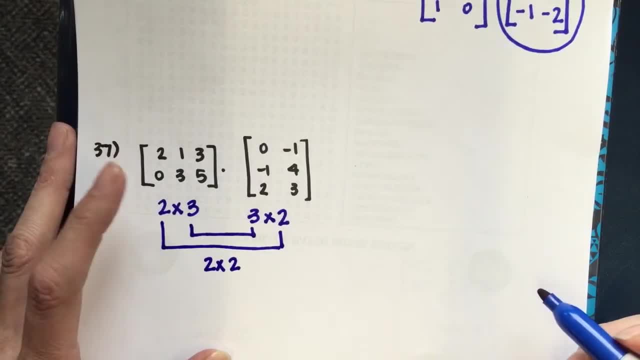 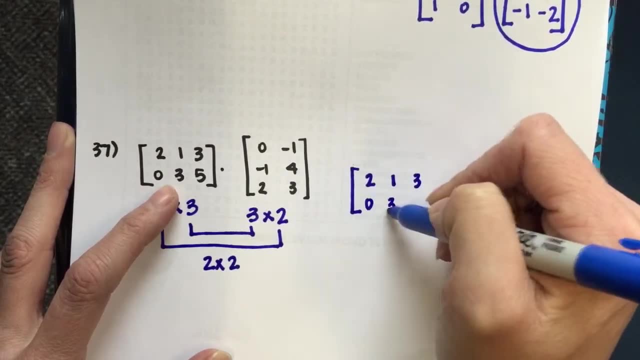 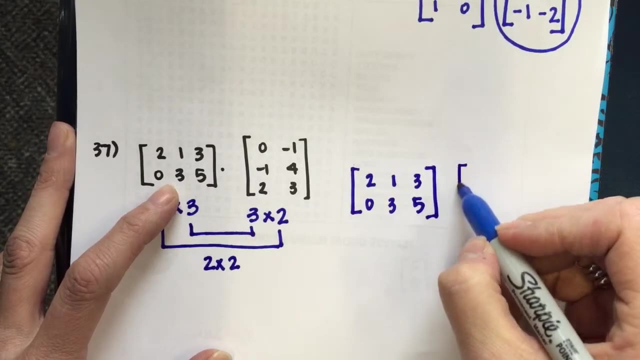 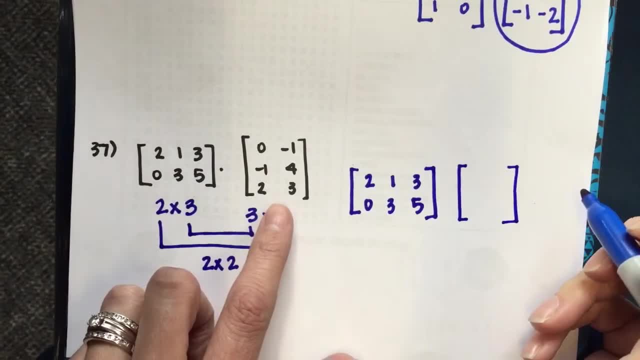 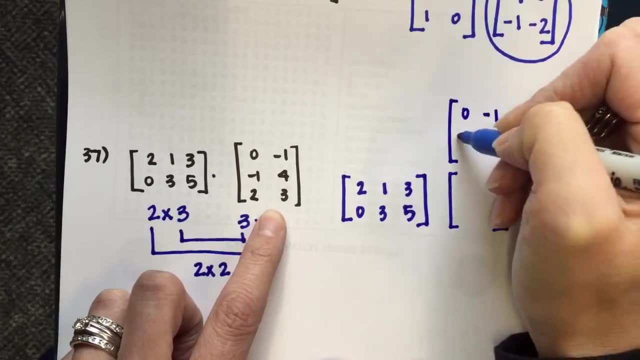 My answer. matrix is going to go right here, That's a 2 by 2.. And then the second matrix I'm multiplying actually goes above my answer. And then the second matrix I'm multiplying Actually goes above my answer. Actually goes above my answer. 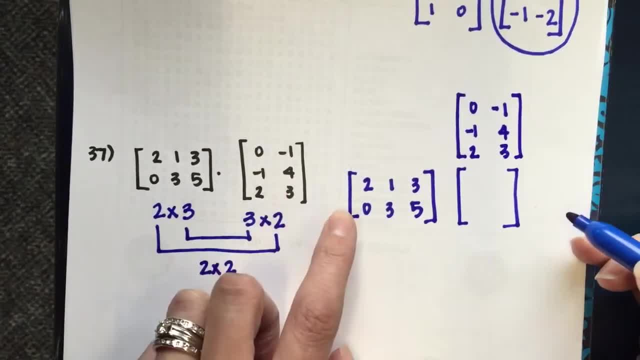 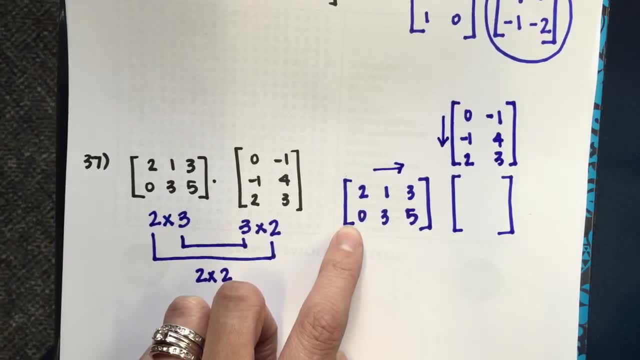 2 by 2.. And this will help you when you line it up. Remember, everything is rows by columns. So I'm going to multiply it And down the rows, And down the rows, these columns. So this first spot on the top left corner, I'm going to multiply the top row. 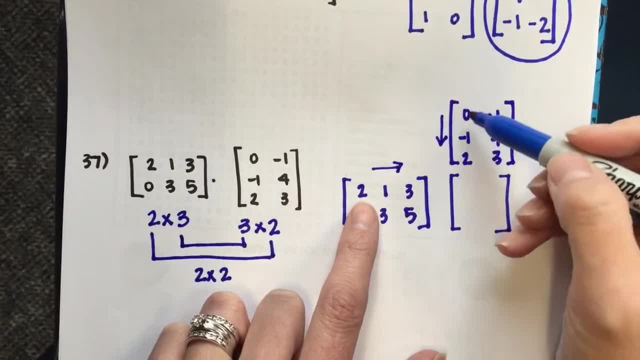 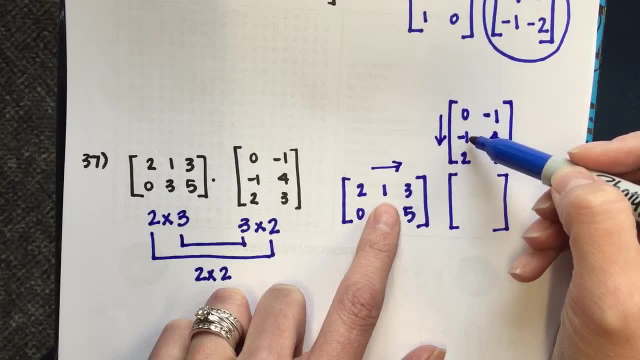 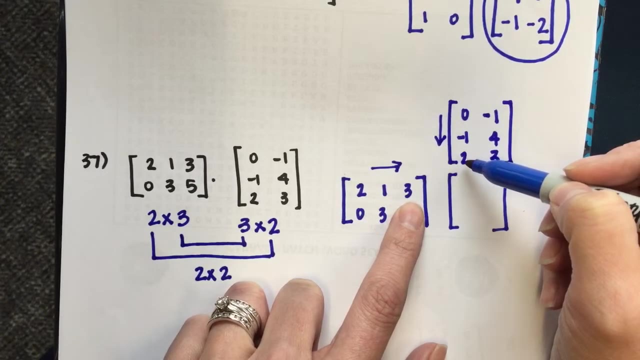 by the left column. Multiply one number at a time from each of them. Two times zero is zero, And then we go to the next number in each. One times negative one is negative one. Then keep going because there's another number in each one. Three times two is six When you get to. 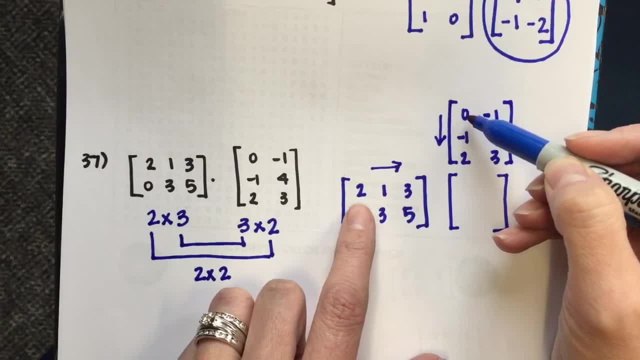 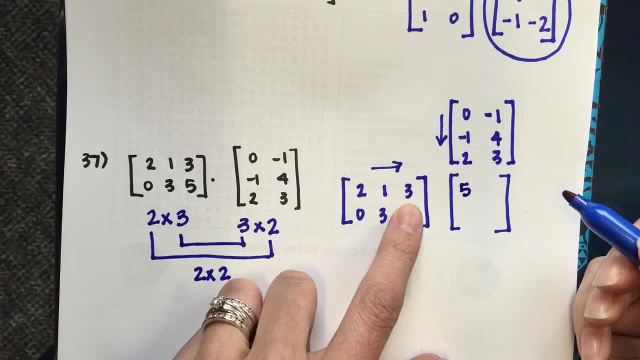 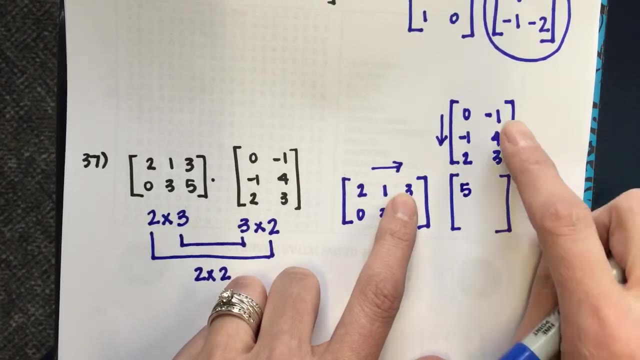 the end and there's no more numbers, then you add them all together: Zero minus one plus six is five, And that's the answer that goes in your product matrix. So now I want to find the spot that's in the top row, right hand side. So I'm going to multiply the top row by the right column.